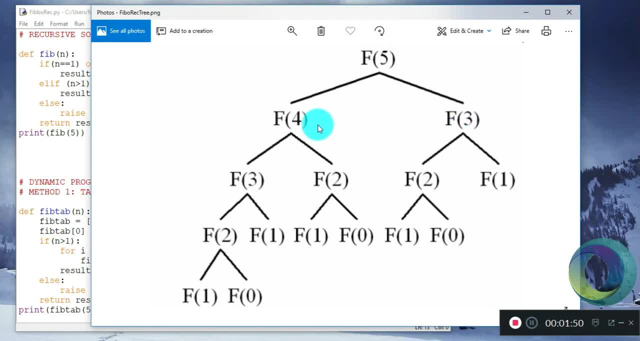 3 are not known, So it again calls f of 3 and f of 2, and this tree grows. The problem with this is that f of 3 is computed twice, f of 2 is computed thrice and f of 1- five. 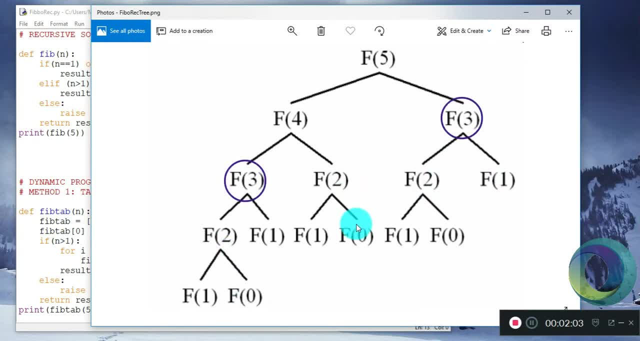 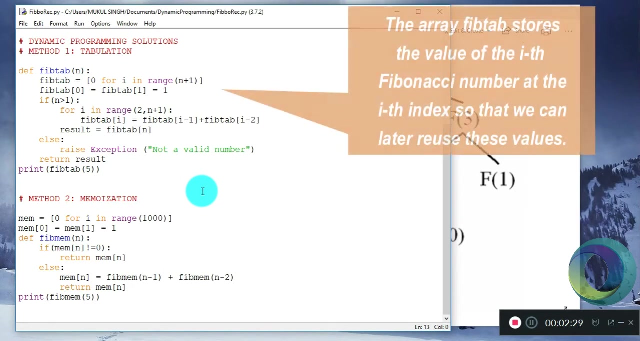 times. This is a waste of computation. What dynamic programming does is it avoids these repeated computations. So instead of computing these values multiple times, we will store them. Let's see how we do that. There are two methods to do dynamic programming: tabulation and memoization. Tabulation: 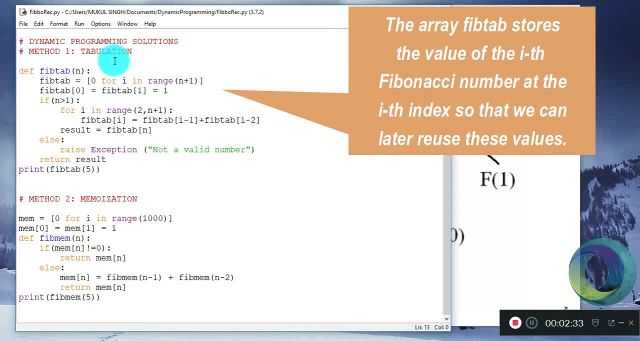 is also known as the bottom-up approach. As the name suggests, we start at the bottom of the tree and move towards the top. giving us the answer. Let's see how it is implemented in this function. 1. We have an array of size n. This array will store the values of the Fibonacci numbers. 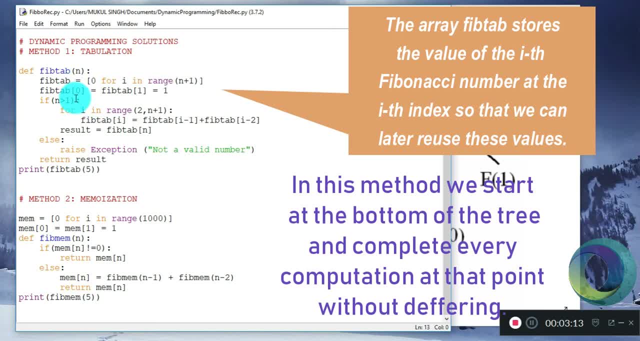 2. As done before, we can see that at zero and one the value is initialized to one. 3. For any value- 1, we will first compute the second Fibonacci number. Now we know the second Fibonacci number, so we will calculate the third. This way we will move up to n. 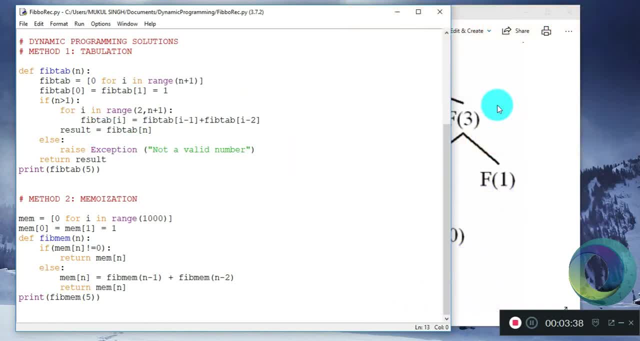 4. Now, why this is better than this tree method is because we have a number called Fibonacci. We have a number called Fibonacci. We have a number called Fibonacci. It is a number and we have a number. We have a number and we have a number. We have a number, We have. 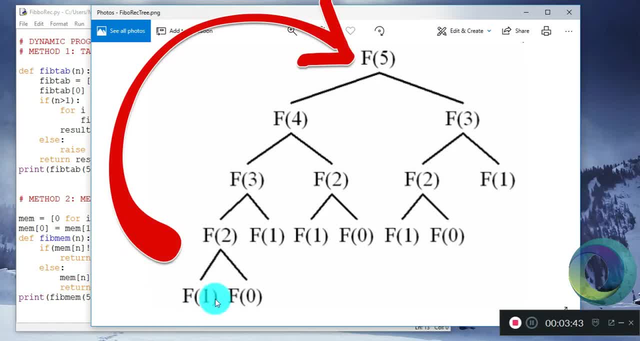 Because from these two we are computing f of 2, then f of 3,, then f of 4, then f of 5.. So no computation is being repeated, Everything is being computed once. Hence it improves the time complexity. 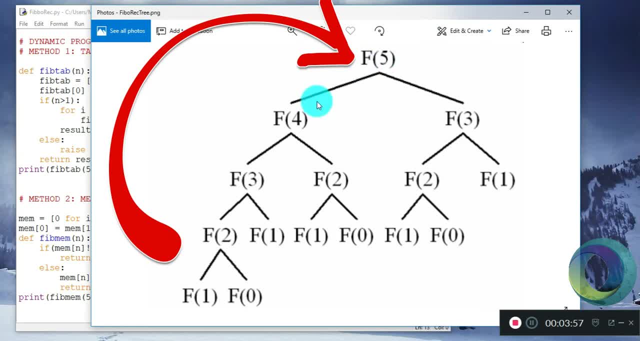 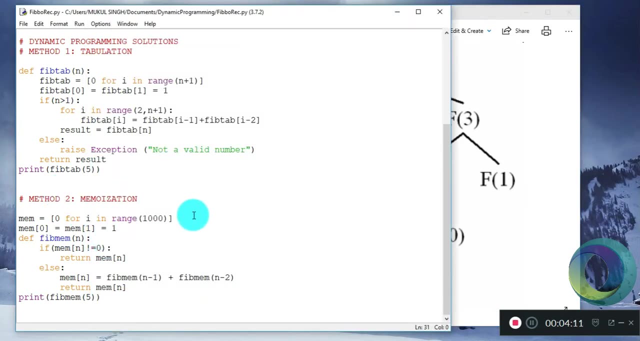 Basically, what we are doing is we are solving the longest branch of the recursive tree. In case of recursion, we have to solve the entire tree, But when we use dynamic programming, we have to solve only the longest branch. The second method to apply dynamic programming is memoization. 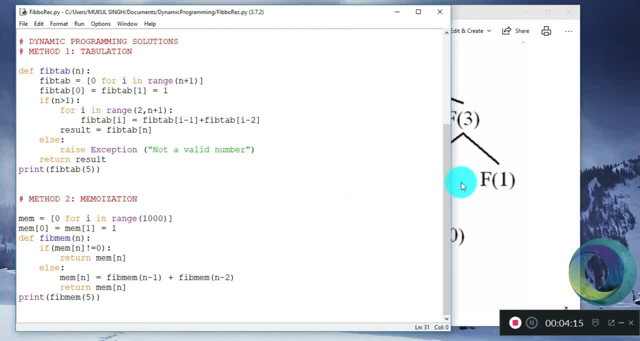 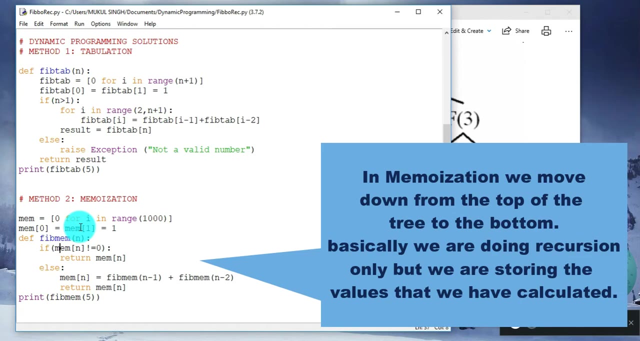 This is known as the top-down approach. In this, we start at the top of the tree and move down to the bottom. For this we need a global array. We have initialized a global array with value 0.. What we are doing in this function, fibmem, is that when the parameter n is passed, 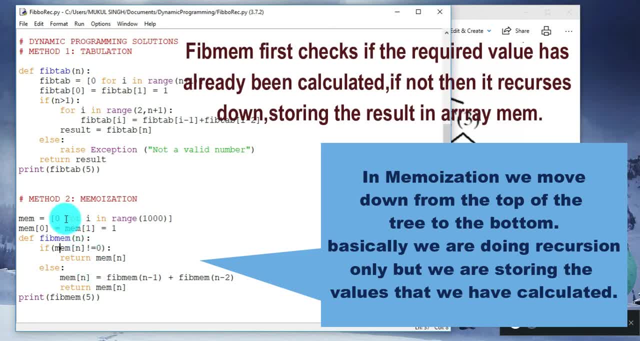 we first check that the value stored at index n in the array is equal to 0 or not. If it is equal to 0, that means that this value has not been changed by us, Hence we have not yet calculated it. But if it is not 0, this means that we have already calculated this value and we just need to return it. 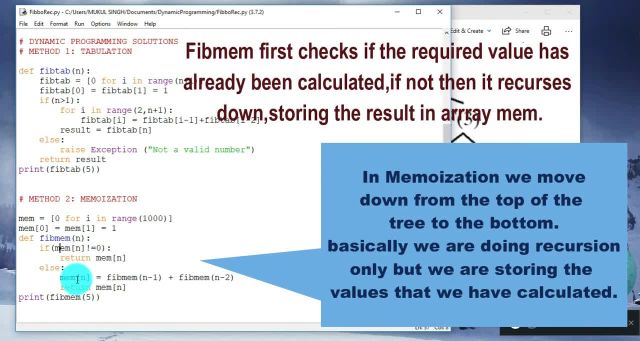 If it is not found, then this function calls fibmem with n-1 and fibmem with n-2 and adds them. This might look difficult, but this is simply what we are doing in tabulation, done in the reverse. Let's see how. 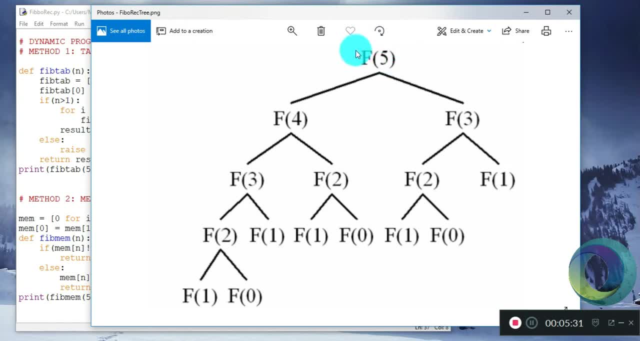 We pass 5 as argument in our fibmem function. Now, since the array does not know the value of f of 5, it will call fibmem function with 4 and the fibmem function with 3.. First f of 4 would be solved. 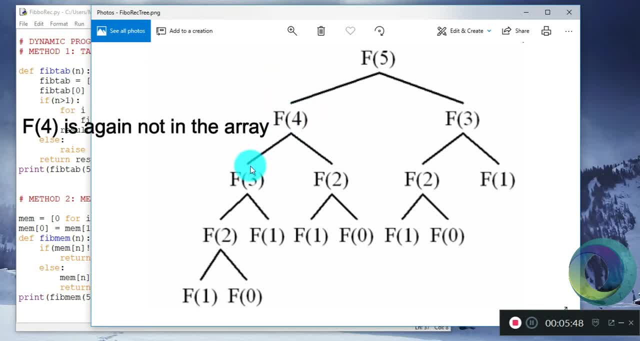 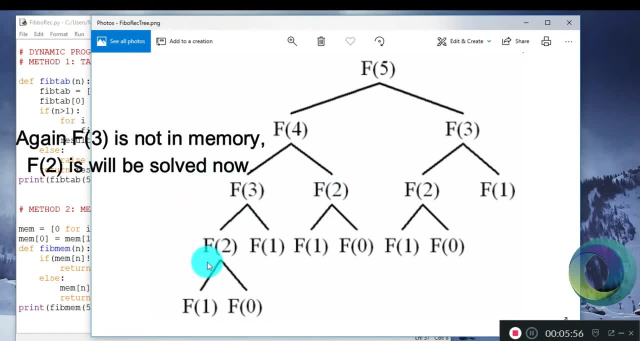 Now again, as f of 4 is not committed to memory, f of 3 and f of 2 would be called First. f of 3 would be solved. f of 2 would be called. If f of 2 is not in memory, f of 2 would be solved and we have the value of f of 1 and f of 0.. 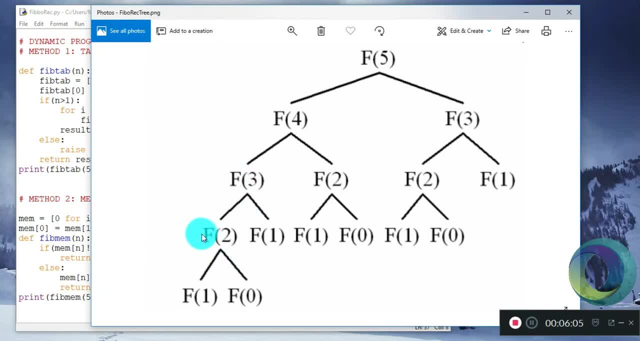 So we get the value of fibmem 2.. Now we get the value of fibmem 3.. Since we have the value of fibmem 3, now we will calculate fibmem 2, but we already have the value of fibmem 2, so we don't need to calculate it. 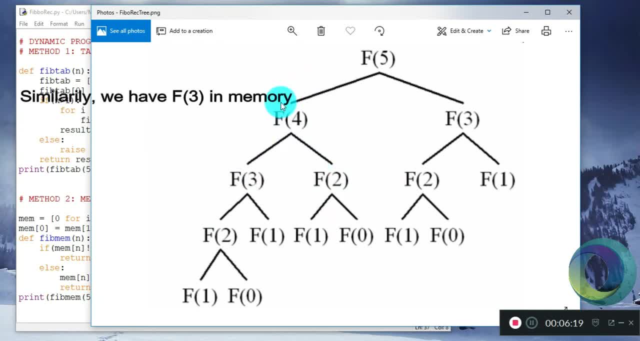 Coming up to fibmem 4,. now we will have to calculate fibmem 3,, but it is calculated here, so we again do not have to calculate it. Hence we get fibmem 5 without repeating. The difference between memoization and tabulation is that in tabulation 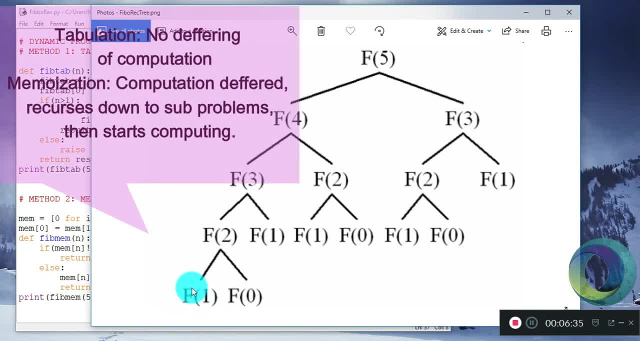 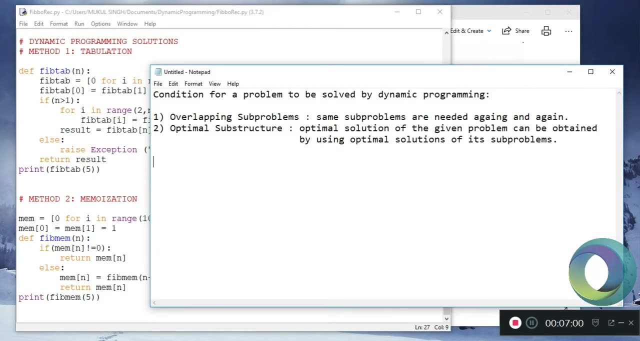 all the computations are occurring at that step only, but in memoization we are deferring the computation. We are not performing the computation at that point, but when the tree starts to open, then we are performing all the computations. You might wonder when to use dynamic programming to solve a problem. 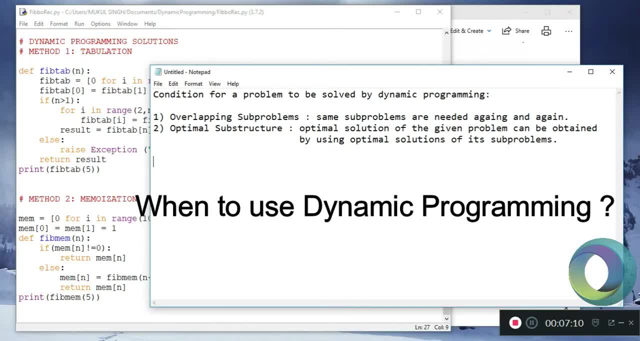 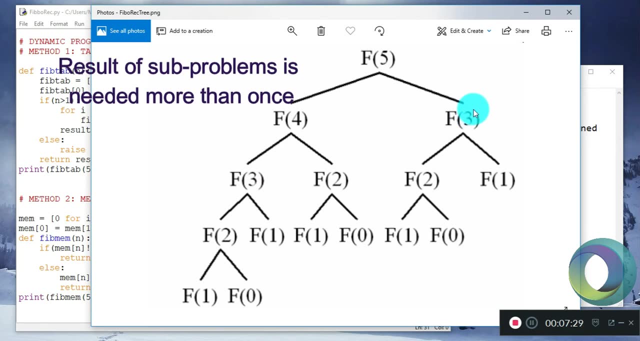 Well, there are two simple conditions to check if a problem can be solved by dynamic programming. The first one is overlapping sub-problem. This means that the same sub-problem needs to be solved again and again. In our recursion tree we saw that f occurred twice and f occurred thrice. 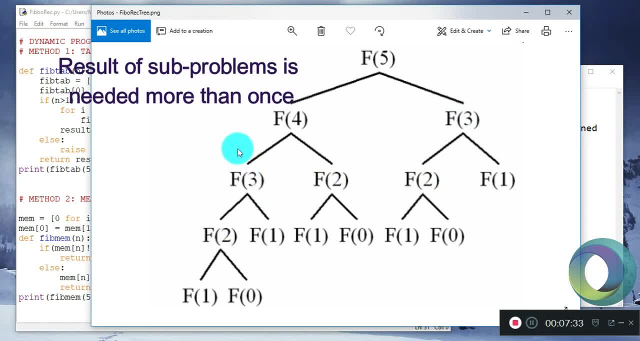 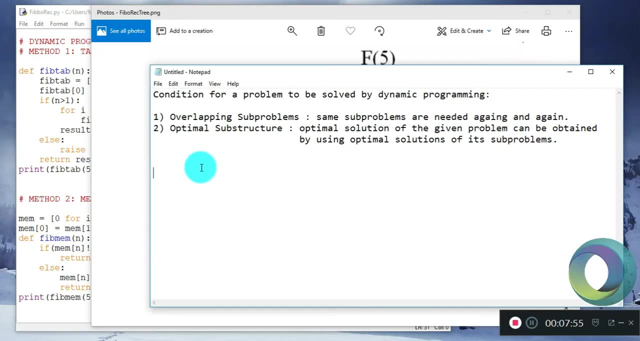 This means that the same computation has to be done multiple times. If f and f would not have been repeated, then remembering the values would not have helped improving the complexity. Second condition is optimal substructure. The optimal solution of the given problem should be obtained by using optimal solution of its sub-problems. 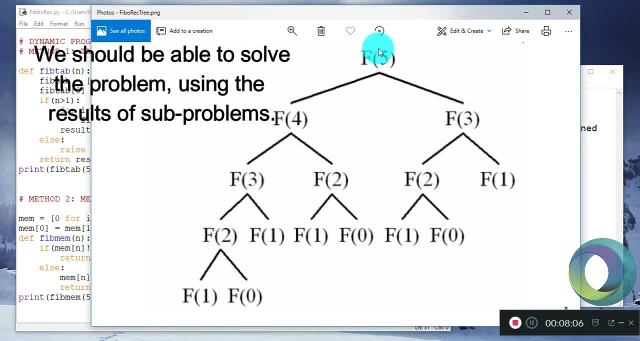 What this means is, like: your problem is to calculate f, Sub-problems are f, f, f, etc. So if you can express f in any expression involving f, f, f, f, f, then the function can be optimally represented. 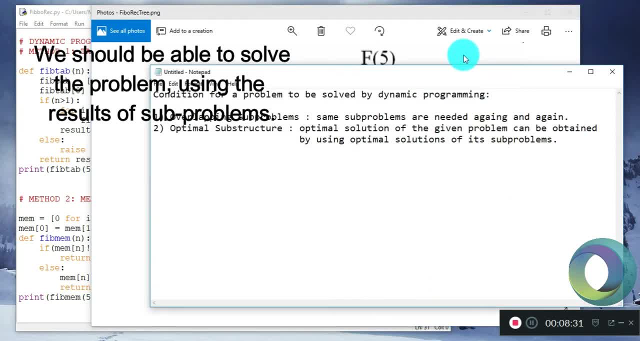 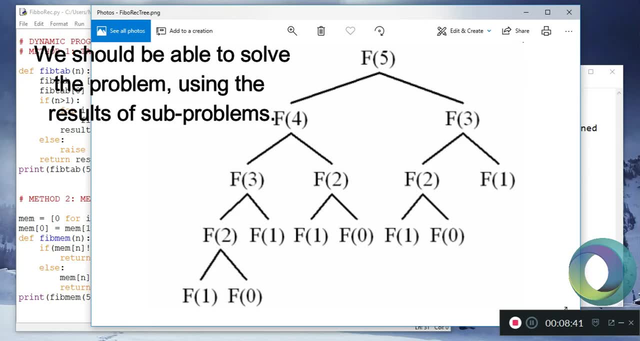 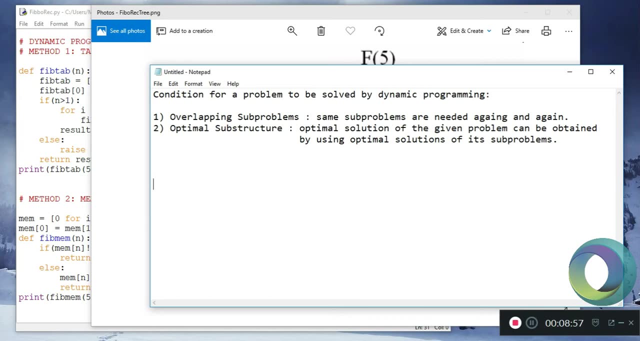 in the form of its sub-problems. If f could not have been broken down in terms of f f, then we could not have applied dynamic programming to this problem. Now you might wonder, now that we know dynamic programming is better, let's compare their complexities. 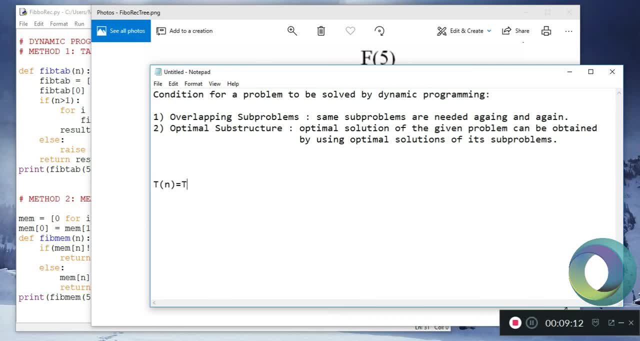 The recurrence equation for Fibonacci numbers is: This is the recurrence equation for Fibonacci numbers. What this means is the number of steps required for n is equal to the sum of the number of steps required for n-1 and n-2.. If you continue solving this, placing the values, 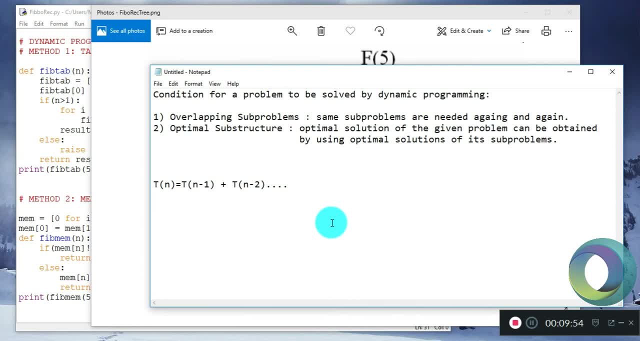 you will find that the complexity is some constant multiplied by 2, raised to the power n. This is known as an exponential time complexity. In case of dynamic programming, we see that since no computation is repeated for the number n, n computation needs to be carried out. 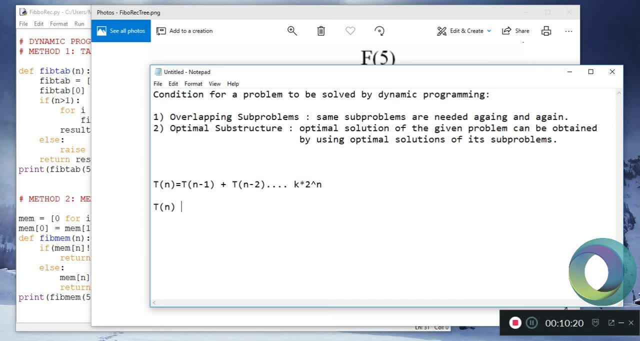 The recurrence equation for this is This: solves to constant multiplied by n. This has linear time complexity. Now, when you have a recursive problem, how to convert it into dynamic programming: 1. Check if it follows the above condition, the overlapping sub-problem and optimal substructure condition.